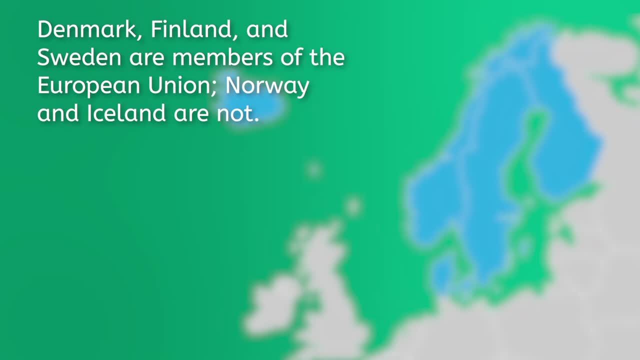 It may surprise many to learn that the nations are all of the same. It may surprise many to learn that the nations are all of the same. Sweden and Finland joined in 1995, while Denmark has been a member since 1973.. Iceland and Norway have chosen not to join the EU. 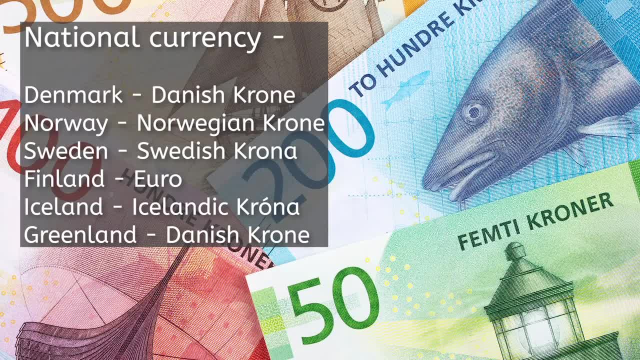 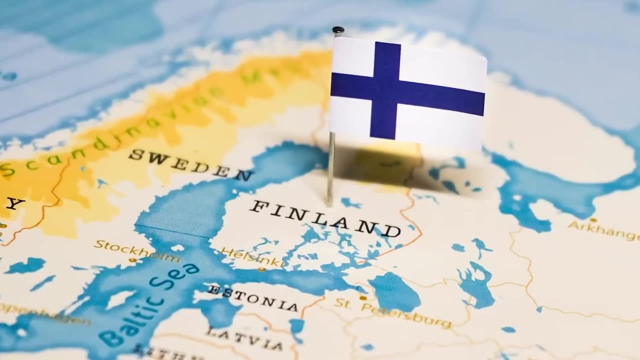 Despite EU membership, Denmark and Sweden use their own currency and not the euro. The krone, or krona, is actually the term for the currency used in Iceland and Norway as well. Only Finland uses the euro as its national currency. Finland is Europe's largest producer of timber. While mining also is a source of revenue for the nation, Norway possesses an enviable amount of natural resources, including petroleum, which accounts for more than 20% of the GDP and about half of the nation's exports. Norway is also the world's second largest exporter of fish, behind only China. 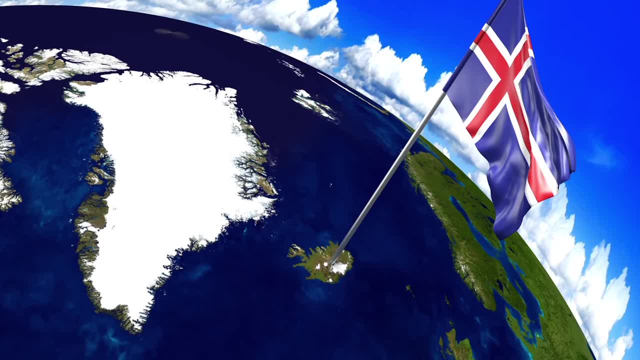 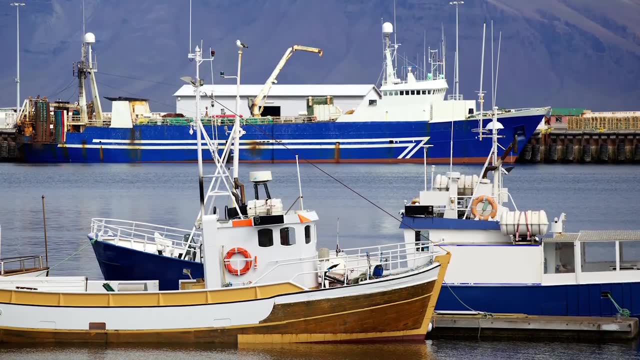 Iceland was, until the 20th century, a fairly poor nation, and much growth has come from diversification of the economy. Fishing is still important, As is exporting aluminum, but manufacturing and service industries have strengthened Iceland's economy greatly since 2000.. 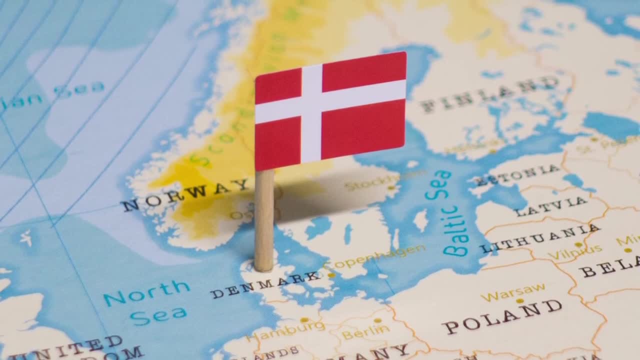 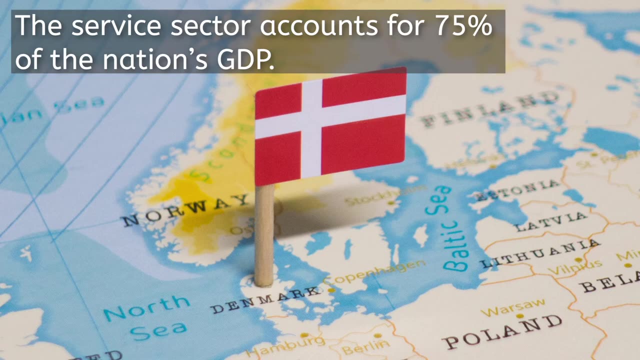 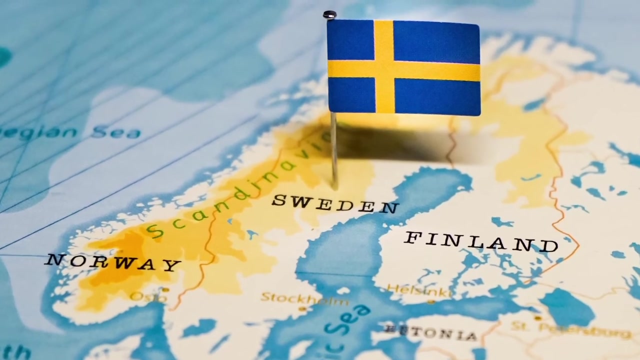 Denmark possesses one of the highest ratios of tertiary degree holders in the entire world, a fact that partially explains how services accounted for 75% of the nation's GDP. The economic structure of Sweden includes a large public service sector with a great deal of export-oriented manufacturing. Recognizable worldwide. Sweden's export-oriented manufacturing industry is one of the largest in the world. The economic structure of Sweden includes a large public service sector with a great deal of export-oriented manufacturing Recognizable worldwide. Sweden's export-oriented manufacturing industry is one of the largest in the world. 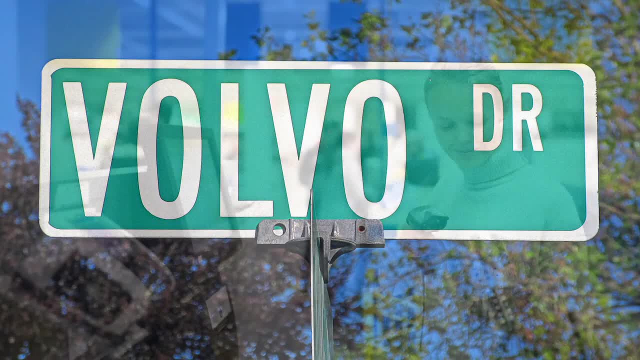 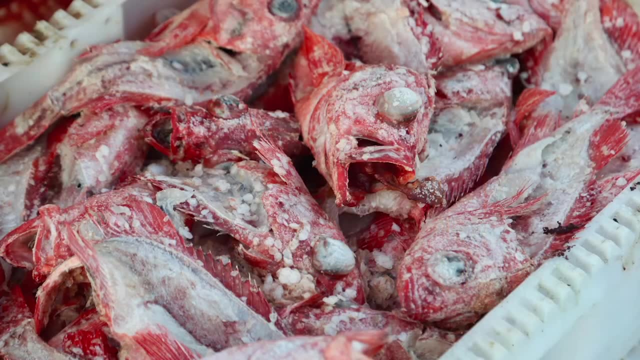 Recognizable worldwide. Sweden's export-oriented manufacturing industry is one of the largest in the world. worldwide corporate icons such as Volvo, Ericsson, Ikea and Electrolux are all registered in Sweden. In Greenland, fishing accounts for more than 90% of the island's exports. 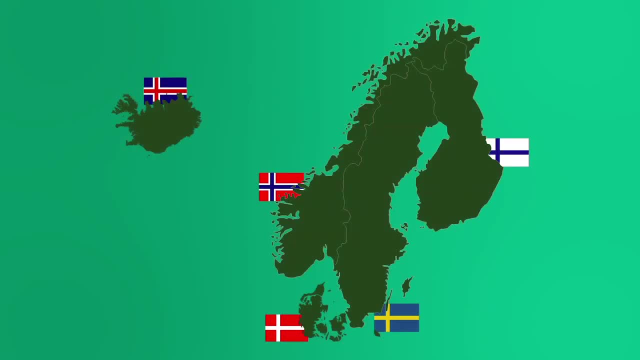 Conclusion: We began today's lesson by asking you a question about the flags of the nations of Northern Europe. We leave now with loads of information about those countries- and a reminder that they, like those in any region, have several commonalities and just as many standards. 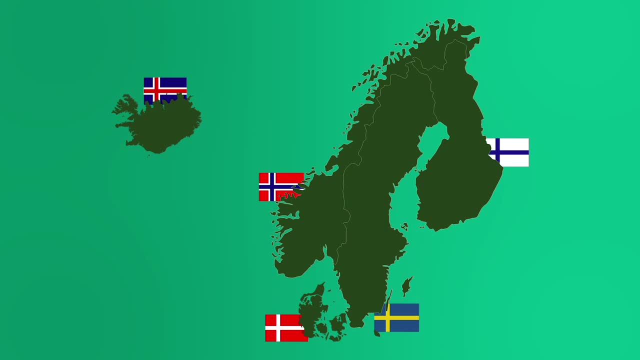 many differences. Until next time, keep exploring. 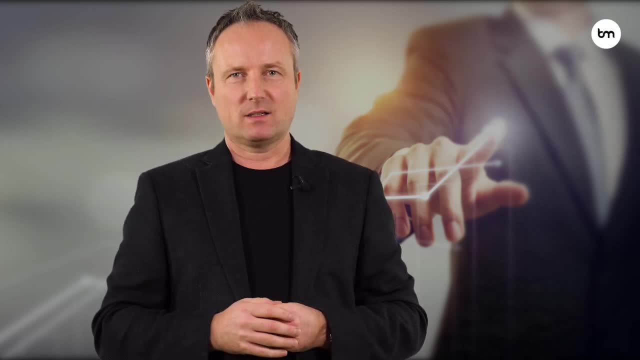 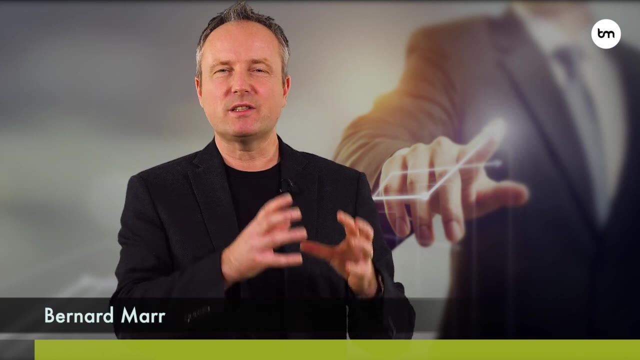 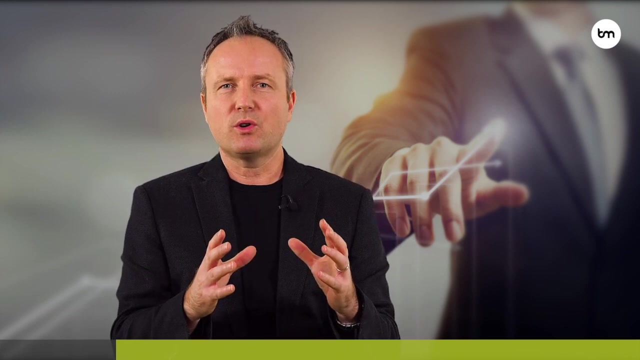 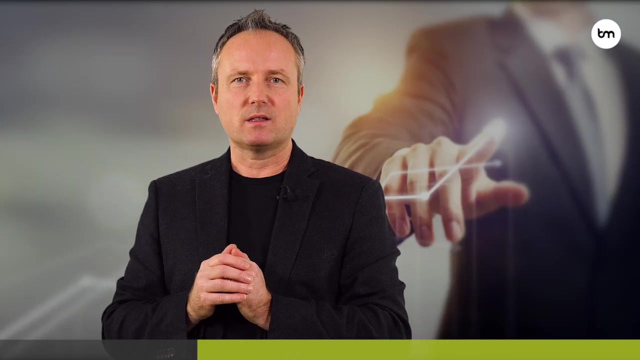 Let's look at augmented reality in just 60 seconds. Augmented reality means overlaying digital images onto the real world to enhance them with digital details. Let's think about Pokemon Go, where we look through our smartphone at the world around us and we get superimposed these digital characters. Or the way we use Snapchat filters to augment our